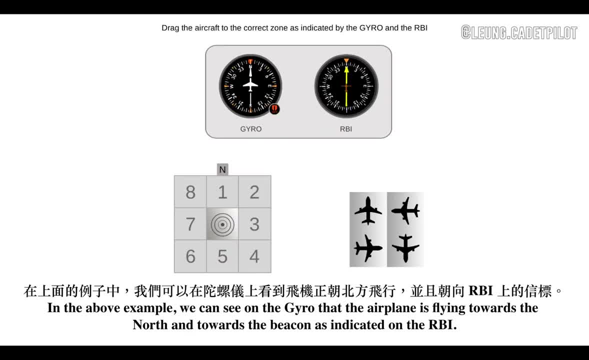 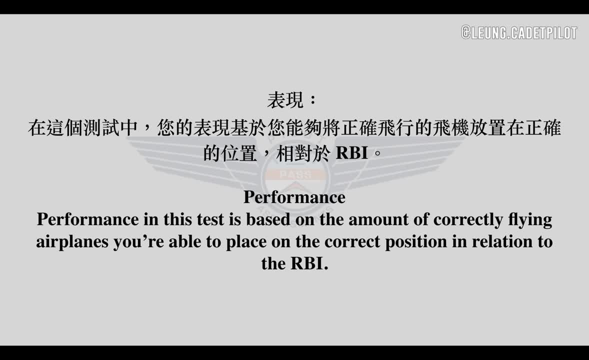 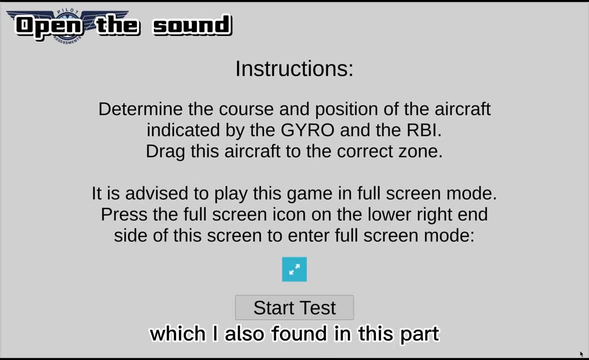 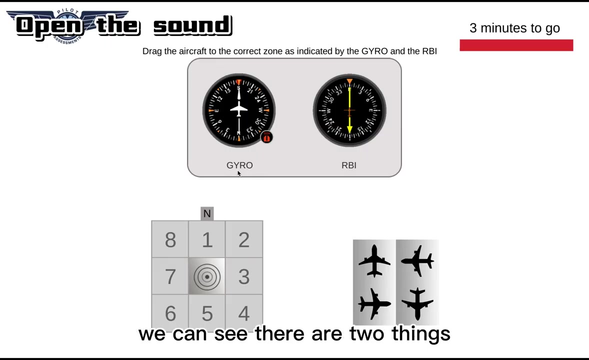 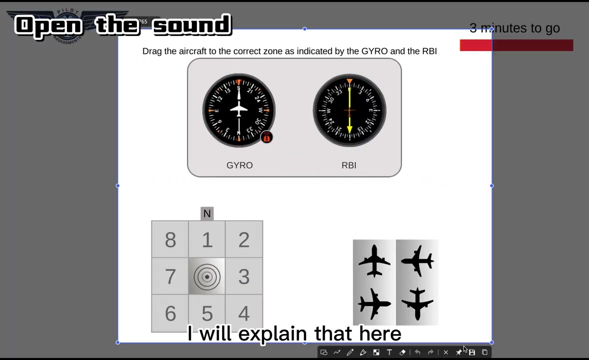 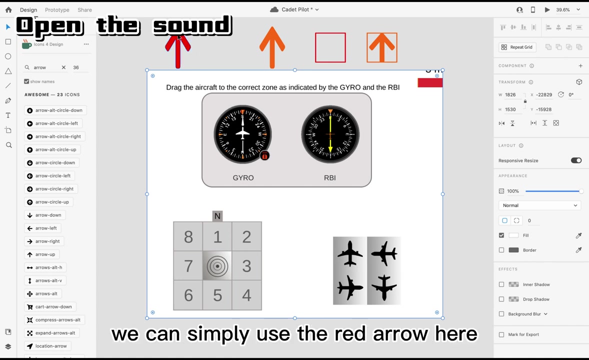 This video is quite difficult, which I also failed in this part last time in my examination. Let's have a look on it. When we press stack test, we can see there are two things: One is GYRO and one is RBI. I will explain it to you. For this question, we can simply use 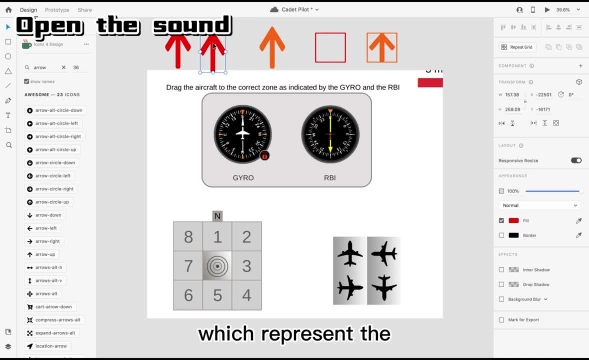 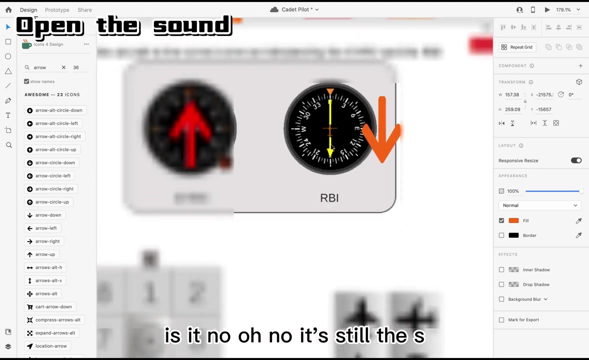 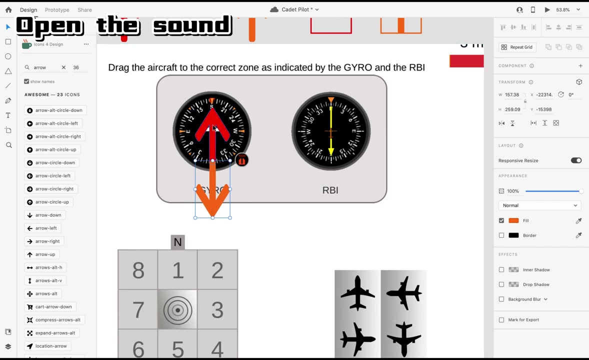 the red arrow here, which represents the airplane weight, and the orange arrow here represents the RBI. In this diagram we can see that the airplane is flying to the S-point, but we want it to go all down through to the S-point. We can simply put these two arrows together. 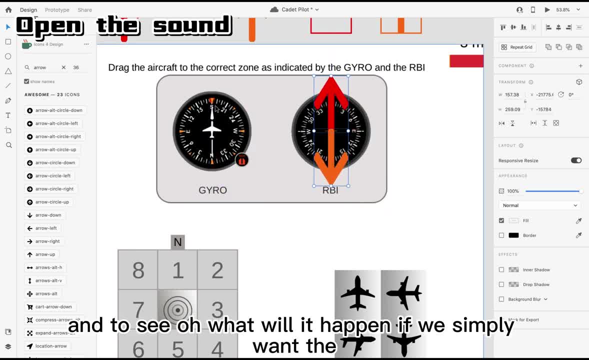 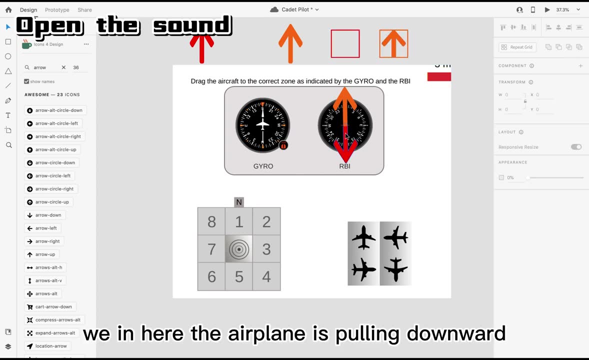 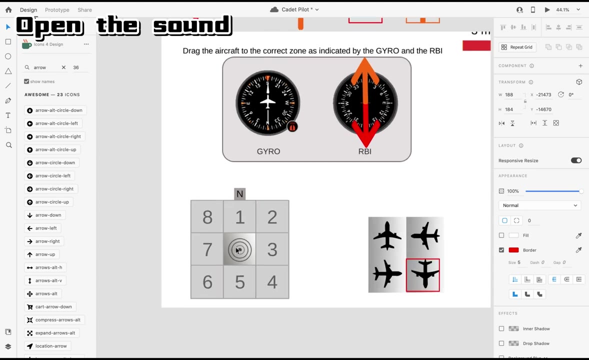 and to see what will happen if we simply point the S-point to the airplane weight. We can see that in here the airplane is pointing downwards, so we need to use this airplane. All we want is to point the airplane to the center point, which is the center point We. 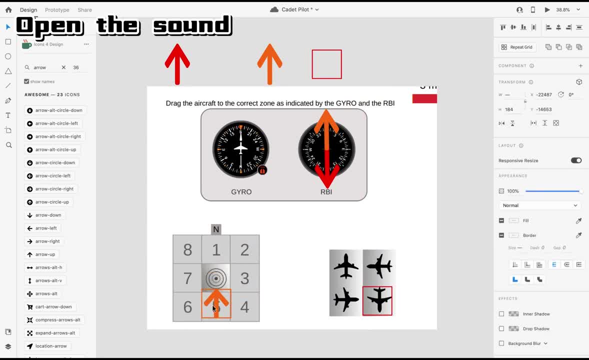 need to point the S-point to the center point, which is the center point, To do that. we point it here so you can see that when the orange point is going to the center point, it means that this one and this one to this one. so we need to put this, everything here. 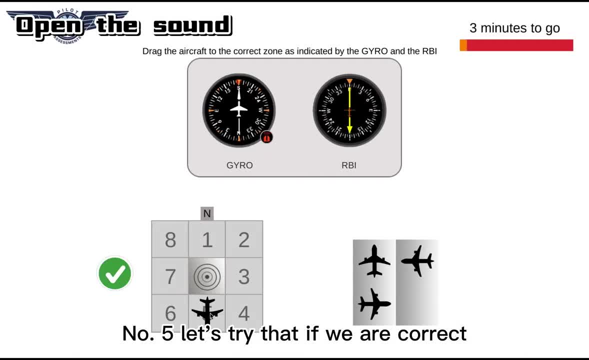 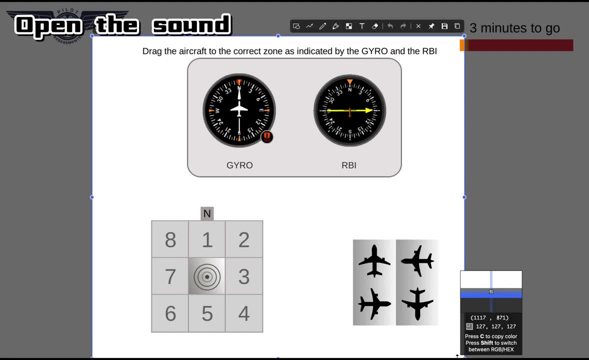 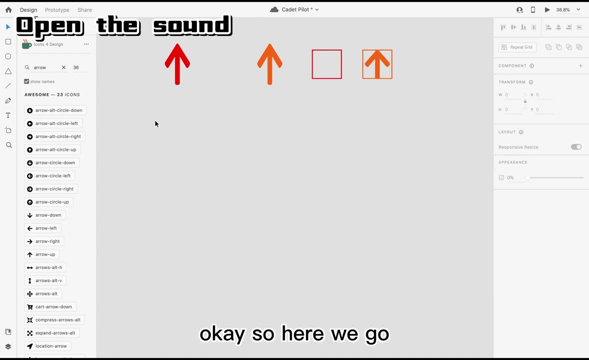 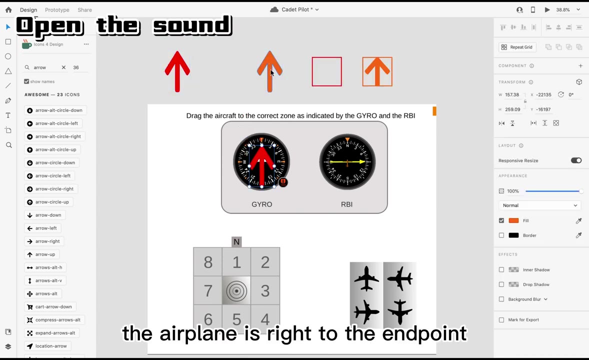 in this number five. let's try that if we are correct. okay, so here we go. okay, another example here. okay, so copy and we can say goodbye to this sample. okay, so here we go. here we go. another example: the airplane is going to the end point, and here the airplane is now going to the east point. so